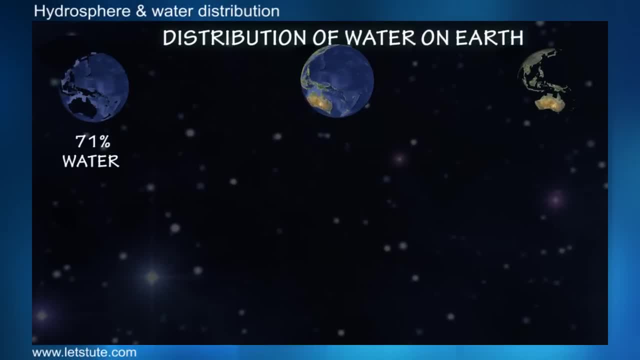 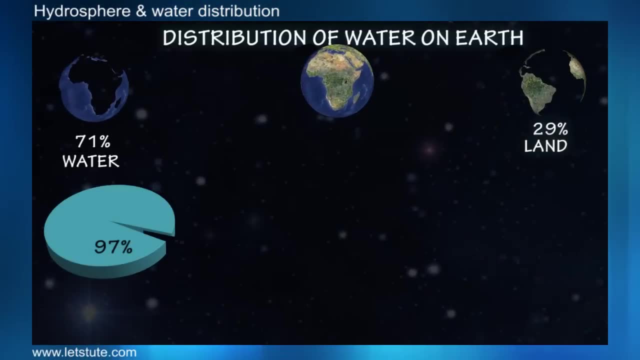 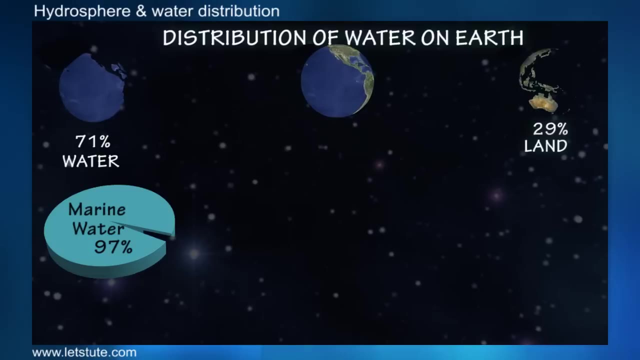 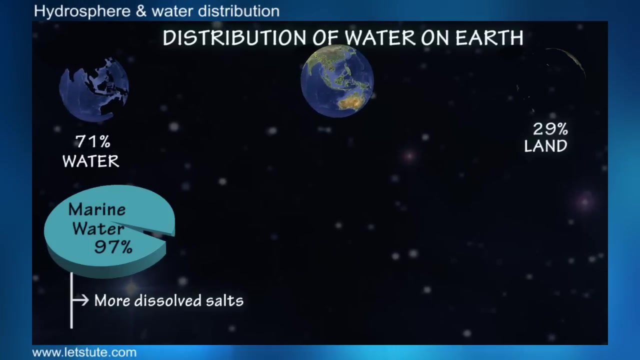 earth is covered with water, and the remaining 29% is land, And around 97% of this water is in seas and oceans, And so we call this water as marine water or saline water, as it has more amount of dissolved salts, and so it's not fit for drinking. And the remaining 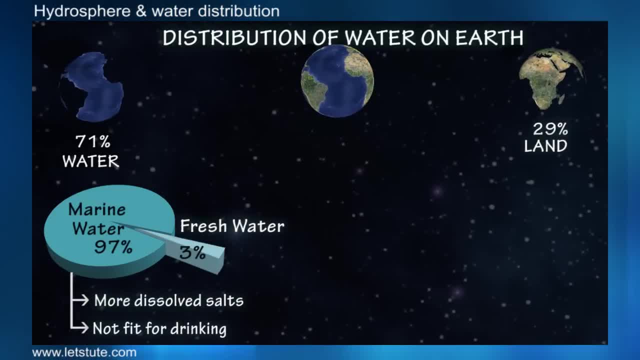 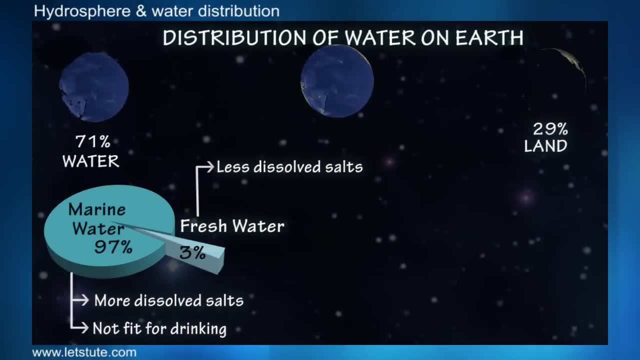 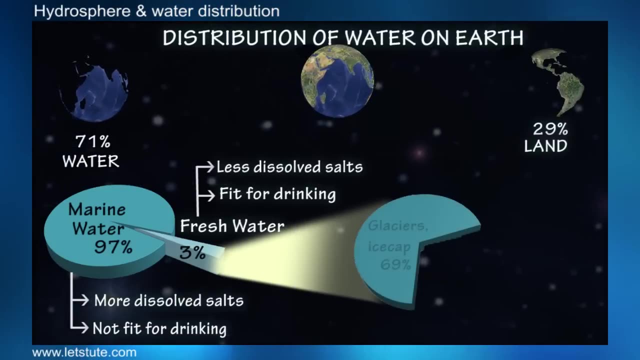 3% is fresh water. Here we call it as fresh water because the dissolved salt content is very less, and that is the reason why it is fit for drinking. And of the total fresh water, major part is locked in glaciers and icecaps, followed by 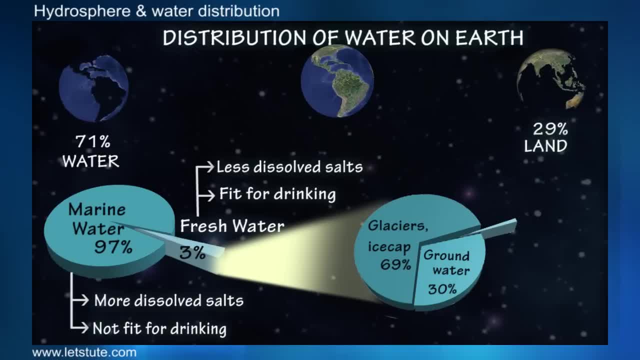 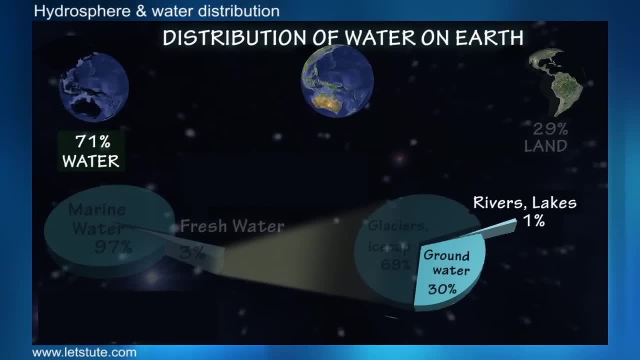 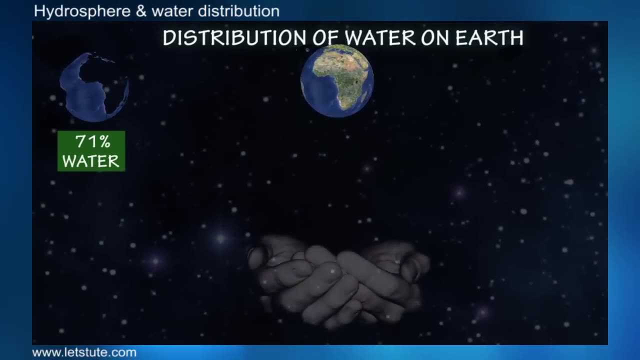 underground water and just a small amount is located in rivers and lakes. So we can compare this small portion of water with the total fresh water Which is available for drinking, With the total water available on the earth, And this is the reason why we must put efforts in conserving water. 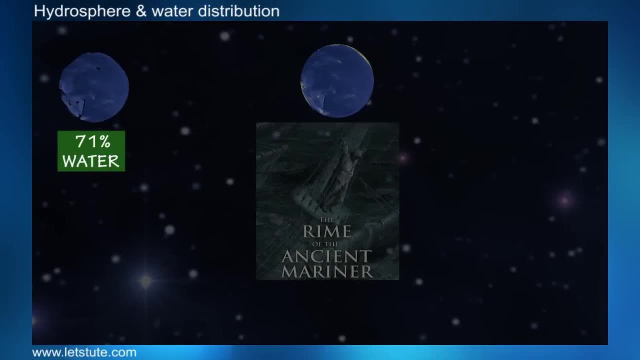 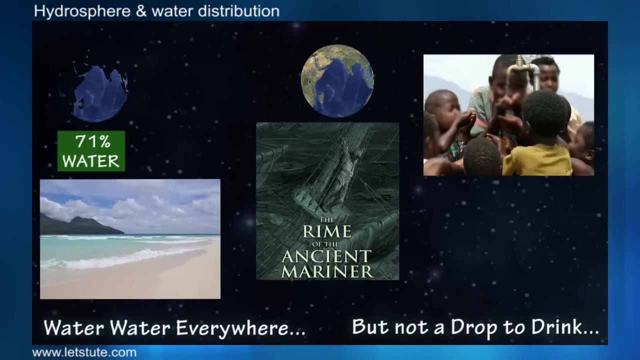 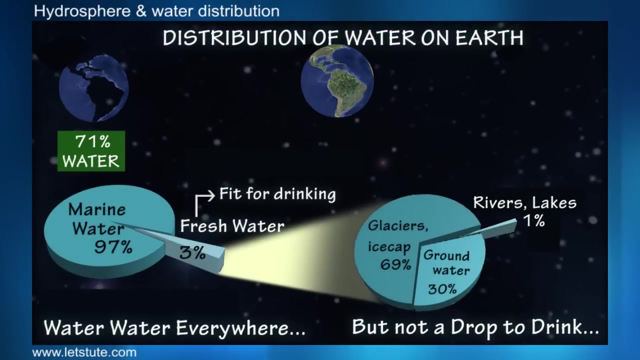 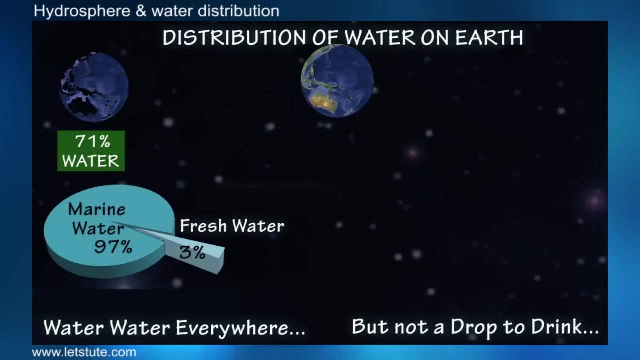 Here I remember the lines from the rhymes of ancient marina water water everywhere, but not a drop to drink. It stands true completely in case of our planet earth, As we have seen just now, that a vast majority of our earth's surface is covered by water, But only a small portion of it is 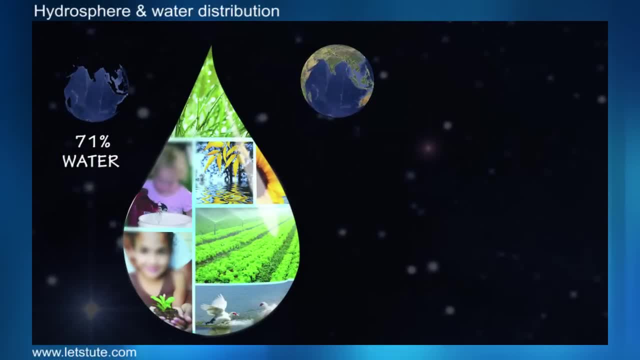 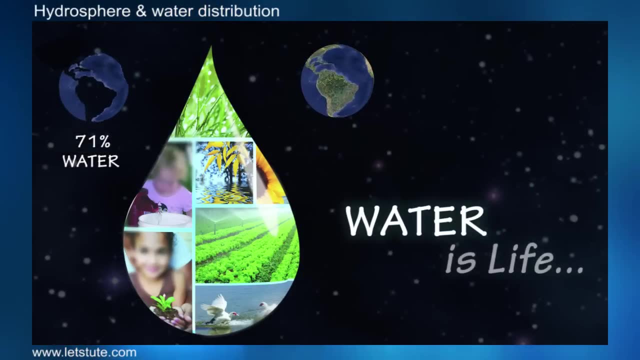 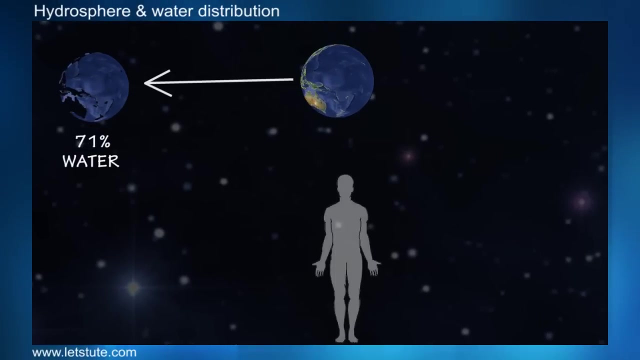 fit for drinking Water plays a crucial role in survival of living organisms on earth. Where there is water, there is life. It is not just the earth that is majorly covered with water, But do you know? water makes up approximately 70% of human's body weight. An average person. 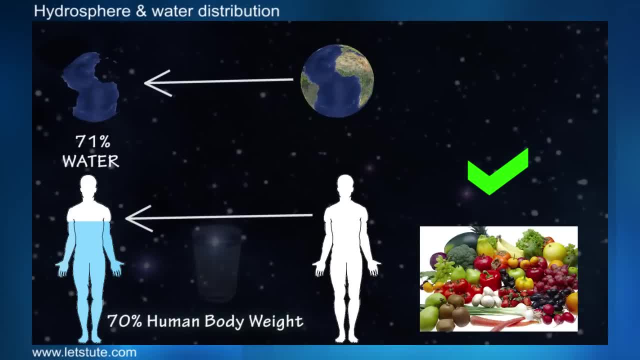 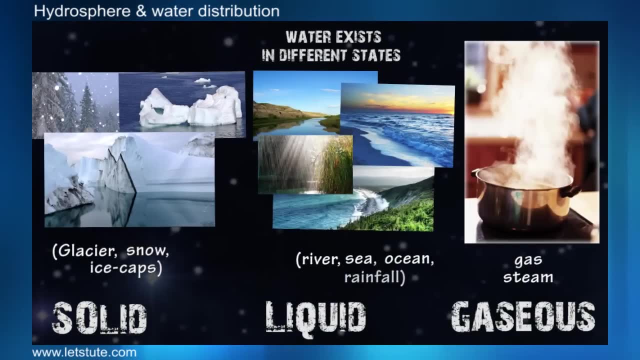 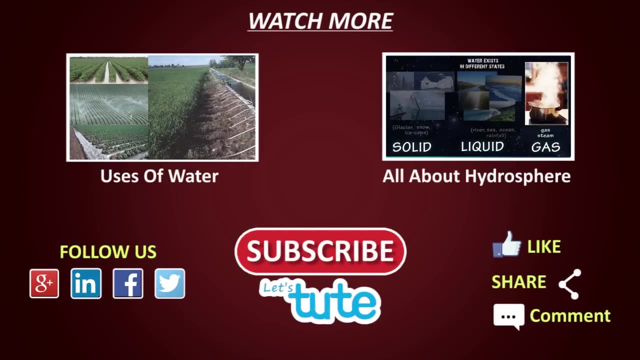 could live without food for nearly a month, But it would just be difficult for us to survive even for a week without water. That's how important water is to human life. So to know more details about hydrosphere, please subscribe If you have liked our session. 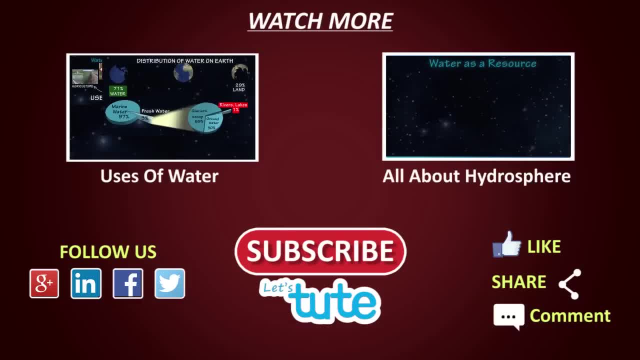 please hit like and do leave your valuable comments. Thank you.